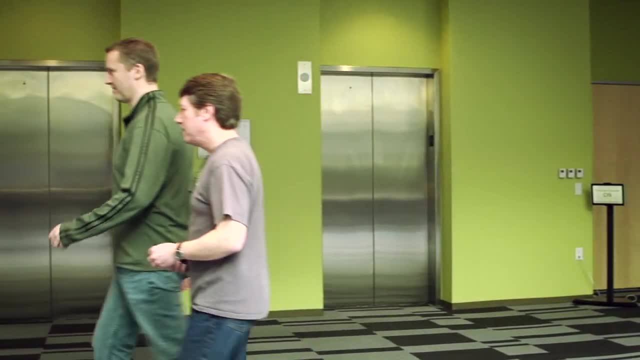 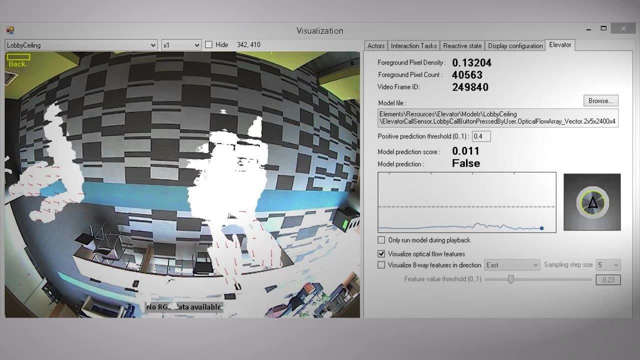 the camera just sees these patterns. It actually relies just on a simple background subtraction, in some sense like it just it's the silhouettes of blobs moving into the scene and based on that information it can anticipate this button will be pushed or this button will not be. 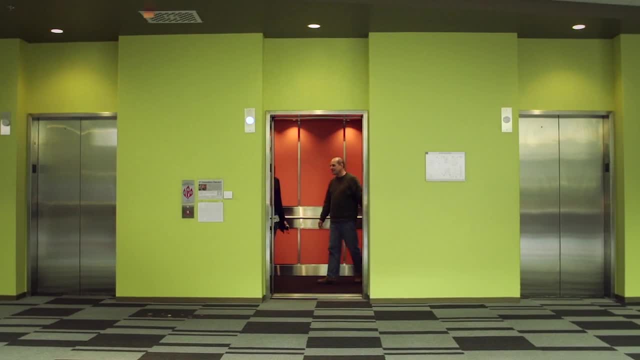 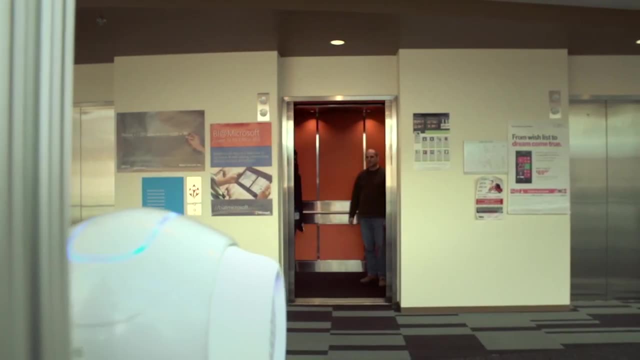 pushed. We use this common framework across these systems, that Mm-hmm That look at some of the same problems but in different settings. It lets us sort of identify in time what are the commonalities here, what are the really core bits, the core. 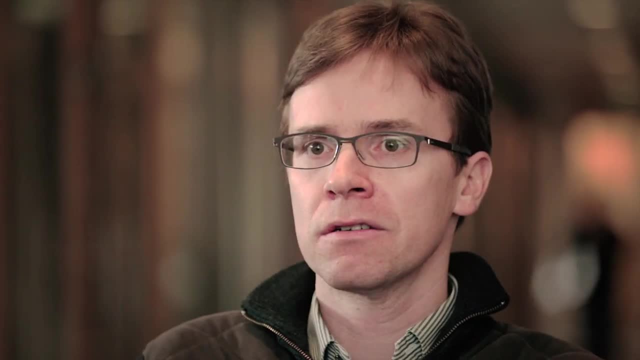 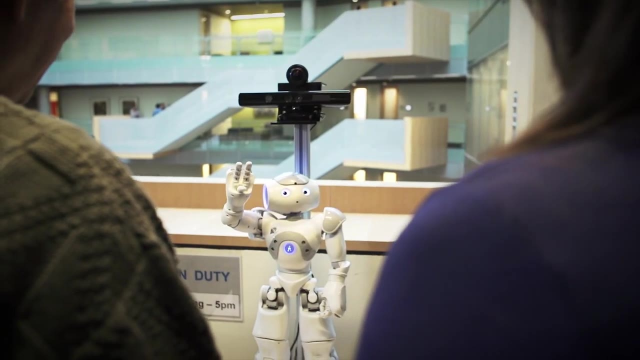 competencies that we need to have in place to generalize across these settings, to be able to do systems that can work well in a variety of settings with people. Do you need directions? Yes, Who or what are you looking for? Eric Horvitz. 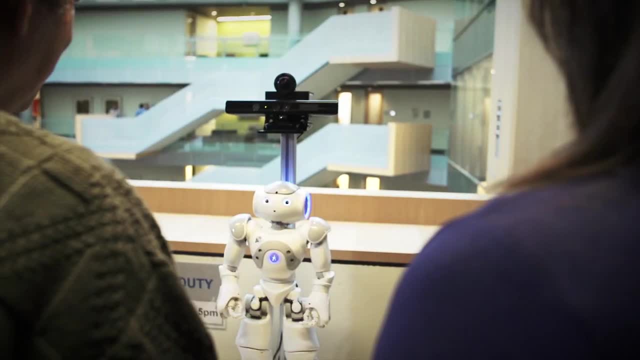 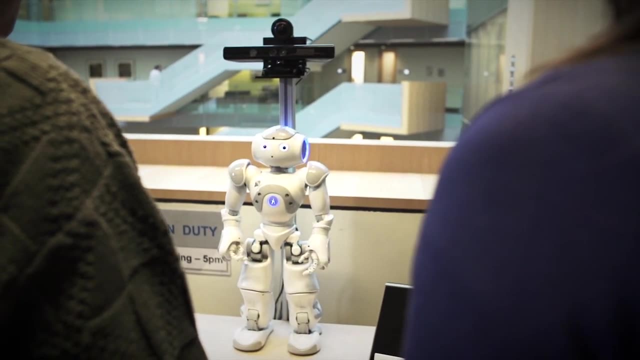 The task of the directions robot is very interesting And it highlights the notion of situatedness Right, The notion of pointing directions in a physical space. understanding where the viewer is and the viewer's perspective on what directions mean. understanding what it means to say you're. 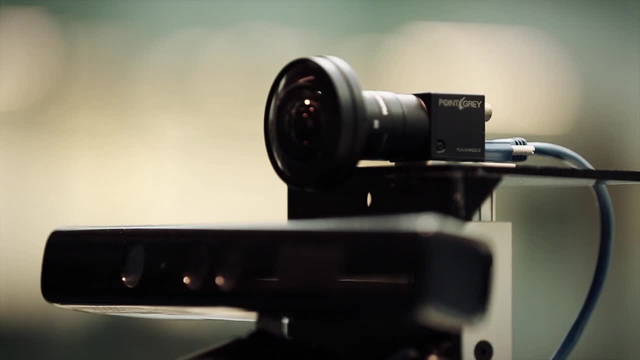 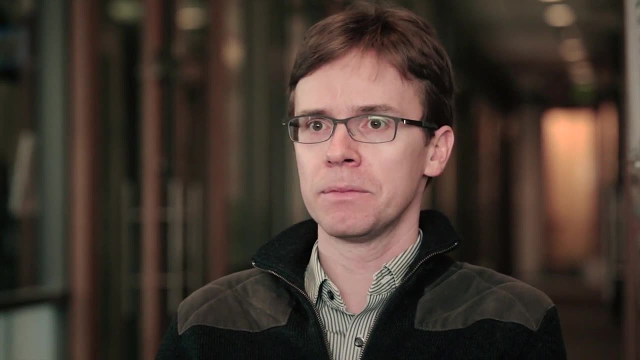 right or on your left. The robot can track multiple participants, so it can track and understand where people are, how far they are, It understands their trajectories and it reasons about that. reason about engagement, which is a basic process that we actually don't think much when we 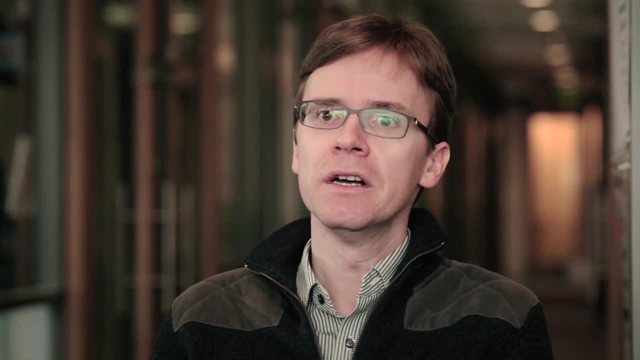 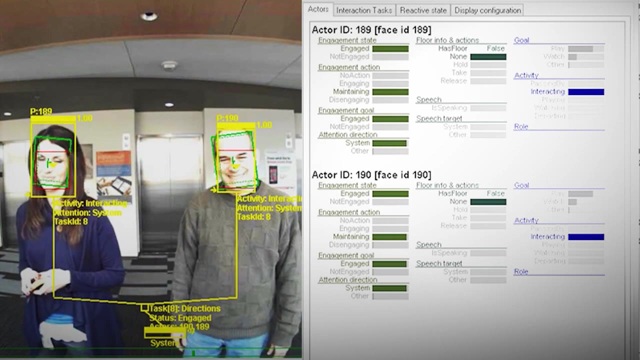 interact, but that happens all the time. How do I know? How do I know I'm still in this conversation with you? A machine will need to reason about all that and we communicate that with various kinds of signals, with how fast I'm approaching you. am I paying attention in that direction? 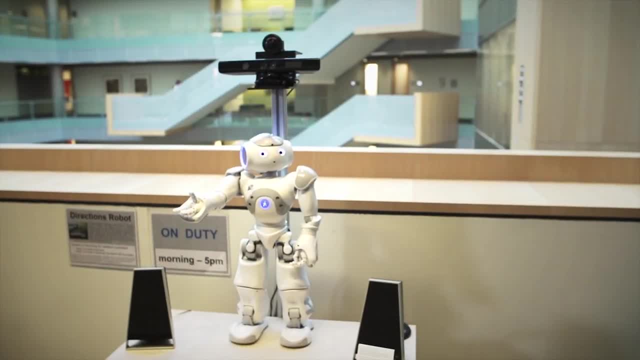 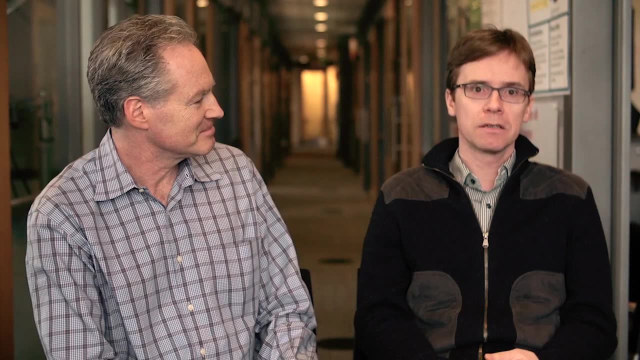 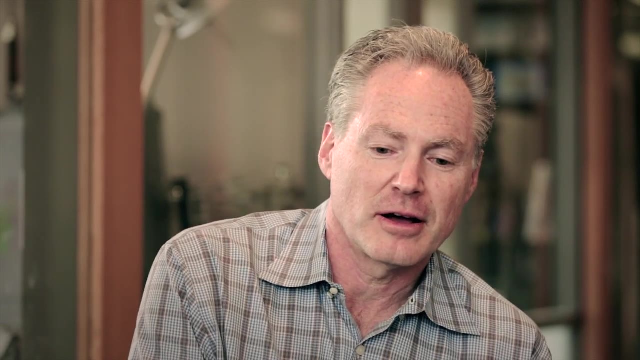 or somewhere else. So trying with sensors using camera and the sound source localization information, all the different kinds of sensors we have. we're trying to make inferences about these aspects. An expert executive administrator working on behalf of someone understands over time the nuances of whether somebody is interruptible or not. 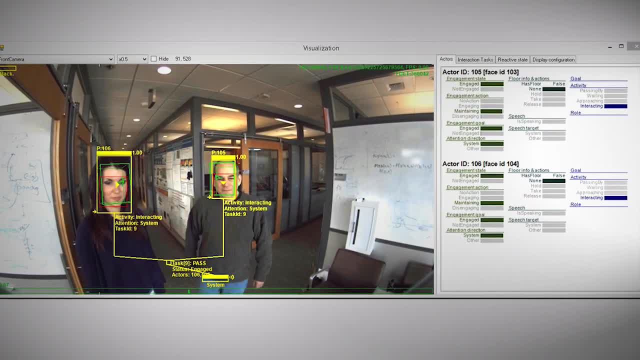 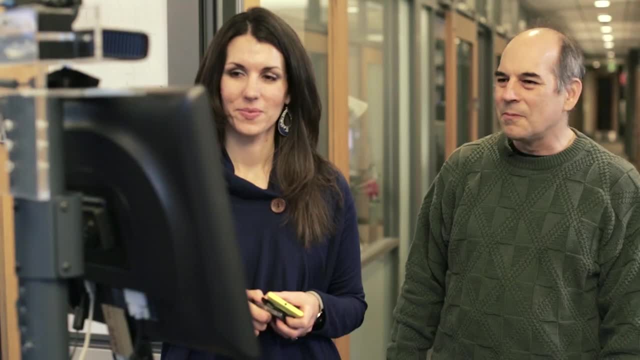 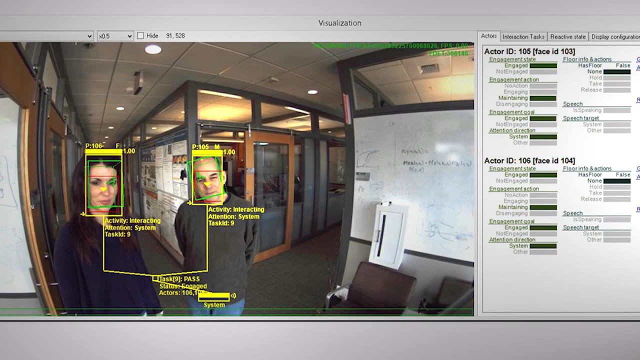 Hi, I was expecting you. The robot told me you were coming. Are you here looking for Eric? Yes, This one really integrates a lot of different knowledge sources. It draws on a lot of work that has been done in the past here by Eric and others on building inference models and.